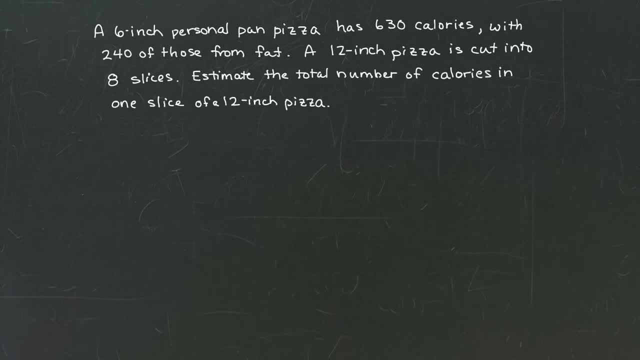 A 6-inch personal pan pizza has 630 calories, with 240 of those from fat. A 12-inch pizza is cut into eight slices. Estimate the total number of calories in one slice of a 12-inch pizza. I think the reason that this problem is so difficult is there's a lot of stuff going on, So let me go ahead and just. 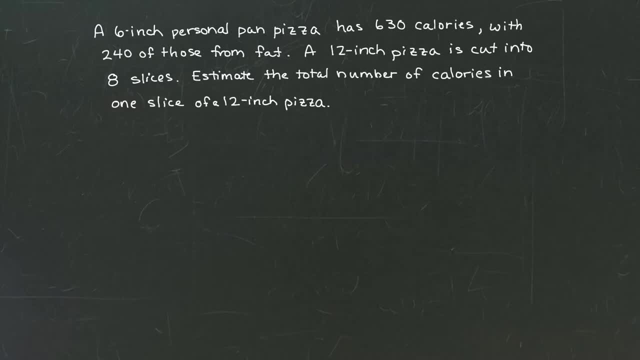 sketch what I need to start to get an overall idea. What I'm starting with is a 6-inch pizza- You know, one of those that you get at Pizza Hut or wherever- those little pan pizzas- and it has 630 calories. 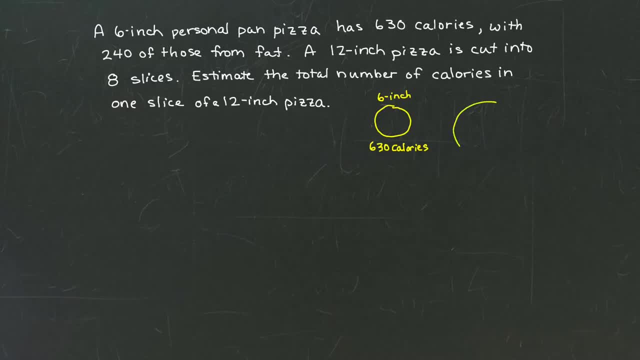 I also have a 12-inch pizza and it's cut into eight slices. What I don't know is: I don't know how many calories are in one slice. So the question is: how many calories are in one slice? Now, do I need to know anything about the fat in each? 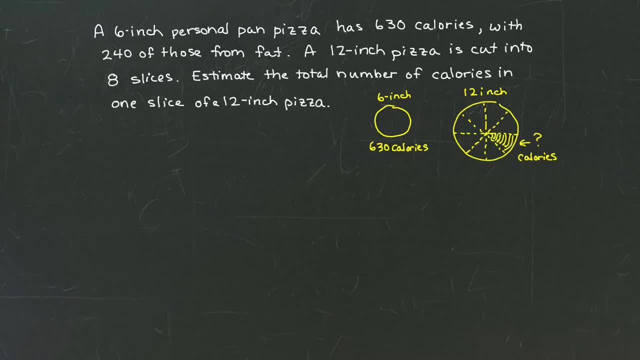 slice of pizza. No, So I actually think this is some superfluous information, so I'm just going to ignore it for now. What I'm going to focus on is: I'm going to focus on the fact that I have kind of a proportion idea being set up. I have a 6-inch pizza compared to a 12-inch pizza, specifically, 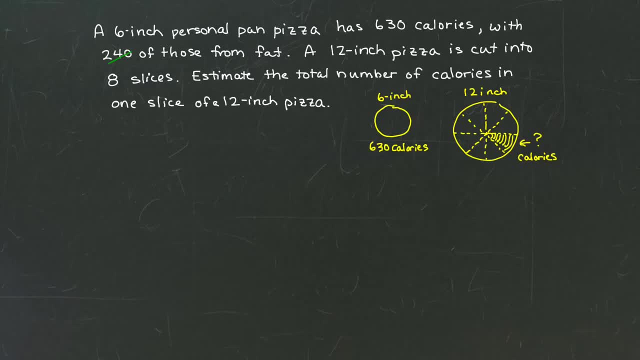 one slice of a 12-inch pizza, and I'm comparing calories to calories. So this is going to be a proportion problem, But it's more in depth than that. When I'm talking about this slice of pizza, I'm talking about a. 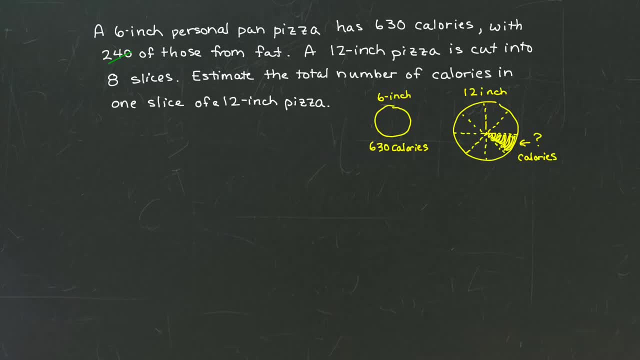 portion of a circle, or in other words, an area. right And same thing over here. When I talk about eating a pizza, I talk about eating this whole pizza or the area of this pizza. So area is also going to come into play. Let's set up our proportion to get us started then. So what am I? 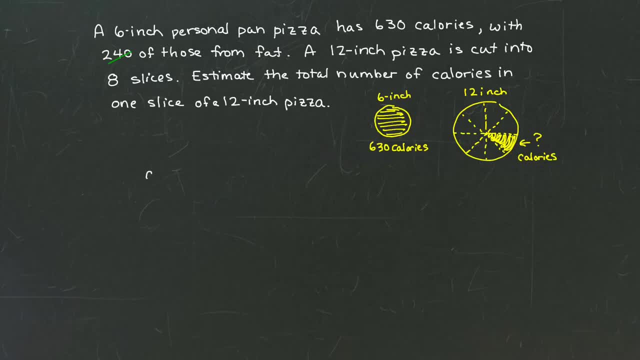 going to be comparing. I'm going to be comparing the area in the whole 6-inch pizza, so the area of the 6-inch pizza, and I'm going to be comparing that to the area of one slice. But I'm going to do it in such a way. 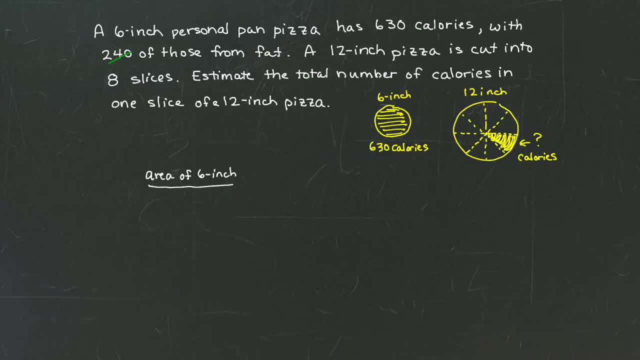 that the area of the 6-inch pizza relates to its calories right in the same proportion or in the same fashion as the area of one slice- which we don't know- And in fact the area of one slice of the 12-inch pizza. 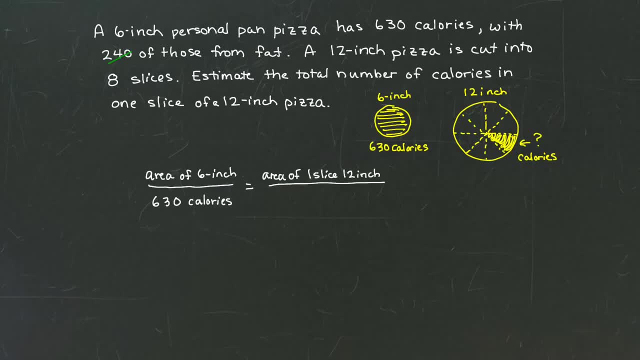 corresponds to the number of calories in that slice. So we have that the area of the 6-inch pizza corresponds to 630 calories, in the same fashion as the area of one slice of the 12-inch pizza corresponds to its calories, which we don't know. 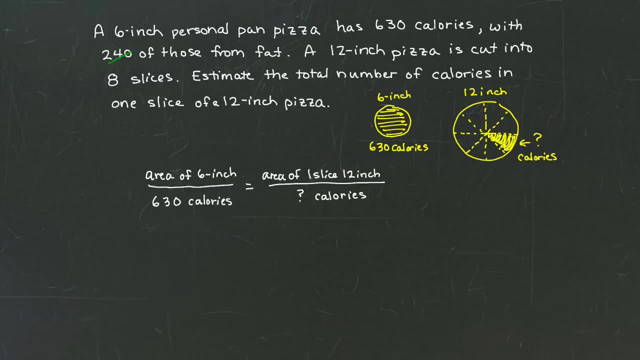 And in fact that's what we're looking for right. We're trying to estimate the total number of calories in one slice. That is our variable x. That's what we're looking for right here. That's what we don't know. 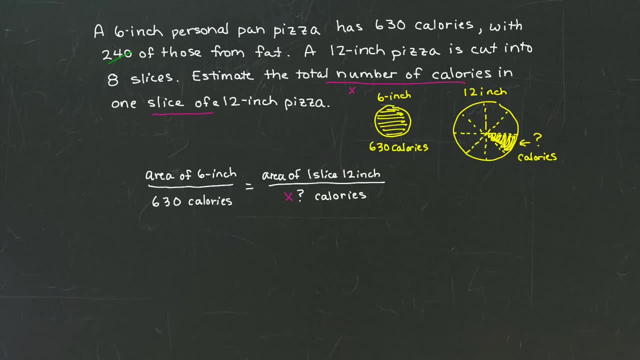 So let's get started solving this. So there are some assumptions I'm making as I begin my problem. The first thing is that these pizzas have the same thickness. okay, That's why we're comparing the area to the area. And the second thing that I'm making an assumption about is that these pizzas are circles. 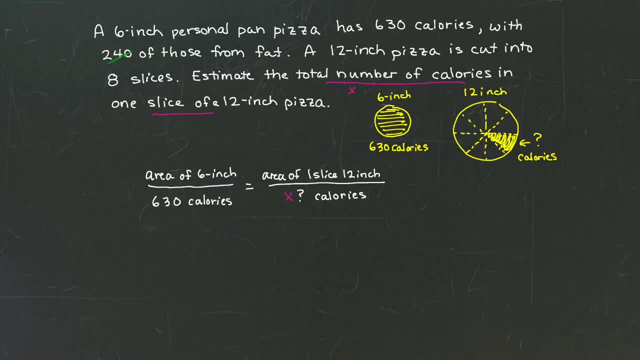 Now, generally the pizzas are circles unless they come in squares, But so we're going to say, when we have a six-inch personal pan pizza, that it's actually a circle. That being said, I need to begin by looking at the formula, then, for the area of a circle. 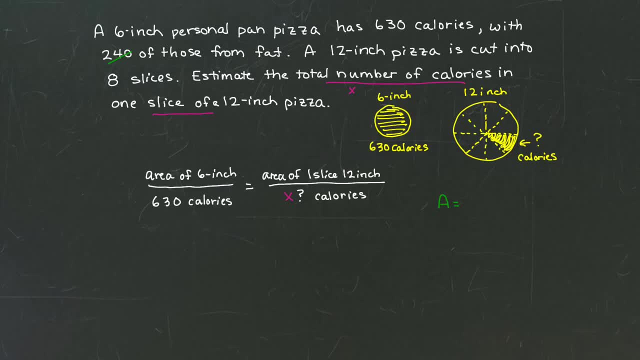 So the area of a circle is equal to pi, our special number, 22 sevenths, or 3.1415.. So pi times r squared, where r is actually the radius of the circle. So if I have a circle and r is the radius, then the area is calculated by taking pi times r squared. 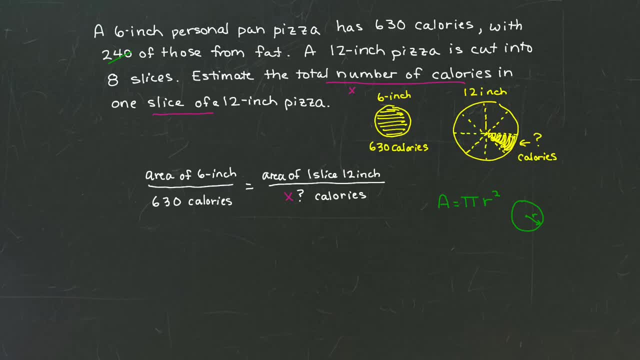 So if I focus and zoom in on my six-inch pizza, six inches describes the diameter, the distance, the whole way across it. And so what would be the distance? What would be the radius for my smaller circle? For my smaller circle, the radius value actually would be three, correct? 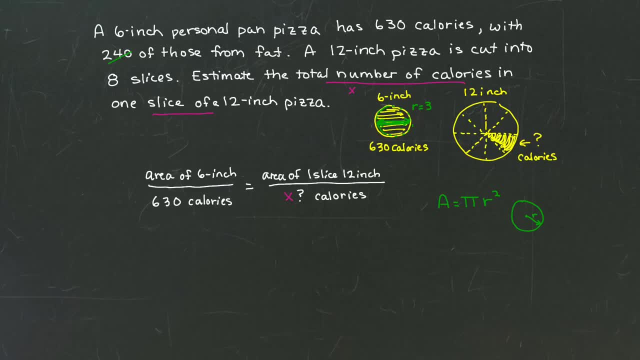 Halfway across six. So that means, then, that the area of my six-inch pizza is going to be simply So. the area, then, of this six-inch pizza- and I'll put it back in my proportion over here- is going to be pi. 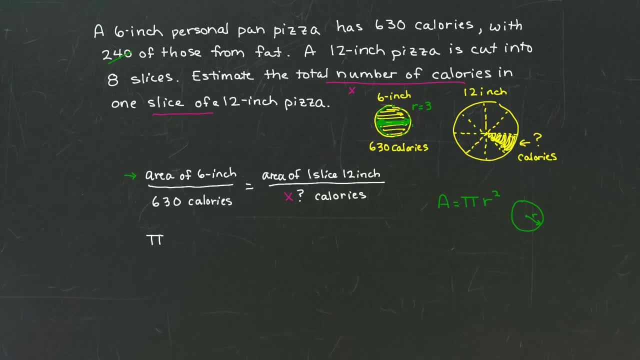 times the radius, which is three inches squared, That's the area for that six-inch pizza, And that corresponds to 630 calories. And it does so in the same fashion. Well, now we have to get the area of the slice of the 12-inch pizza. 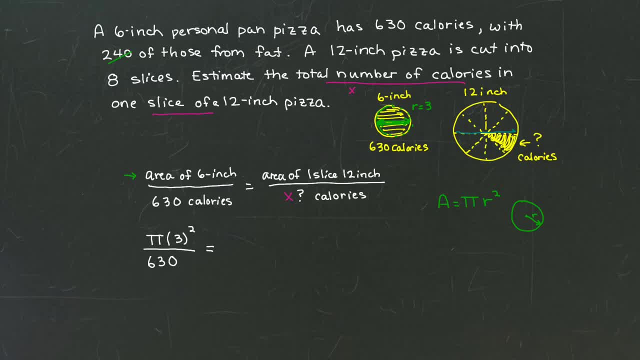 Looking at my 12-inch pizza means The whole way across is 12 inches And so if I want to get the radius which is halfway across, that's going to be six inches. So the radius on my bigger circle is six inches. 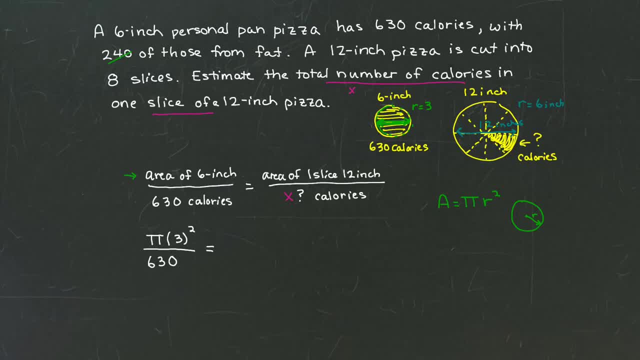 But I have a little more work to do over here. to get the area of one slice I have to take the area of that 12-inch pizza. So that's going to be pi times the radius squared, or six squared. but then I only want one-eighth of it. 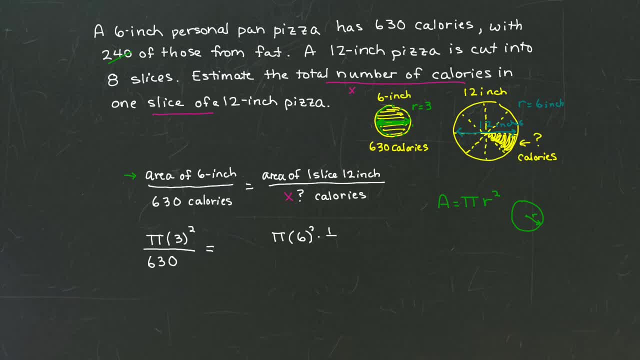 So I'm going to have to multiply this by one-eighth. So I'm going to take pi times six, squared times one-eighth. That gives me the area of one slice of the 12-inch pizza And that corresponds proportionally To the area of the six-inch compared to 630.. 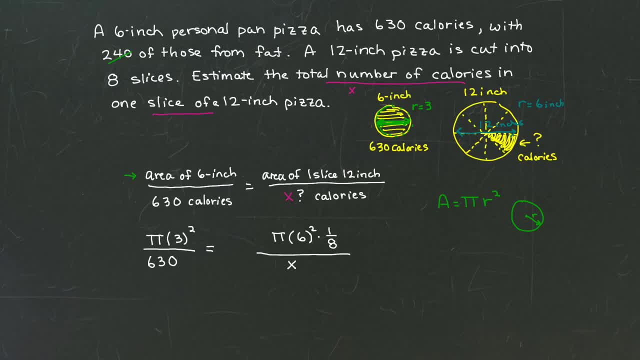 Now we don't know how many calories are in this slice, so I'm going to put an X. We're just about finished. We have our setup and that's the most difficult part. We have that pi times three squared, or three squared, is three times three, which is nine. 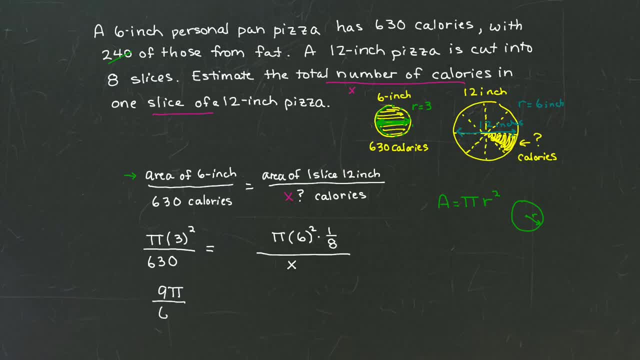 So we have that nine pi corresponds to 630.. In the same way that pi times six squared times one-eighth corresponds to X. So what is that numerator? Well, let's see: Pi times six squared, Six squared is actually 36.. 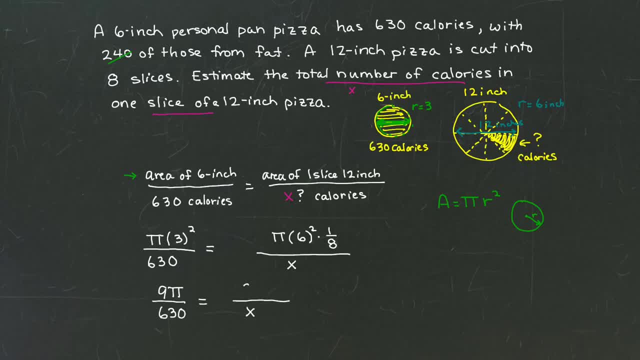 So we have 36 times pi, times one-eighth in our numerator, divided by X. Now we could do some simplification, We could reduce our fractions down, And I actually think that's the way to go. So let's go to a new screen and let's type what we have so far. 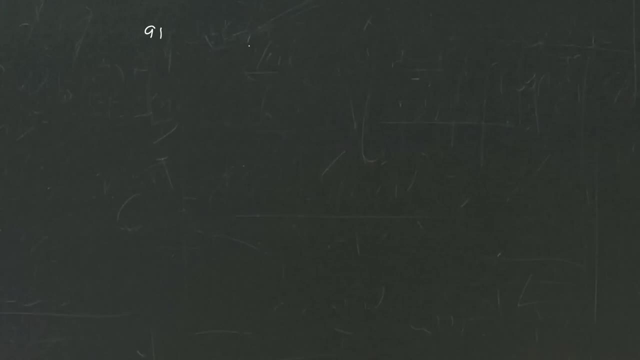 We have nine times pi divided by 630 equals 36 pi times one-eighth all over X On the left side. if we reduce, we're going to take nine and 630. And I notice that nine divides into nine and it divides into 630.. 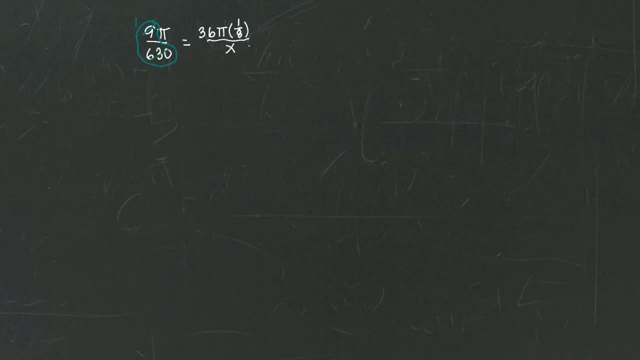 So nine goes into nine one time and nine goes into 630 70 times. So on the left side I actually just have pi divided by 70.. Now on the right side I have to do a little thinking as well. 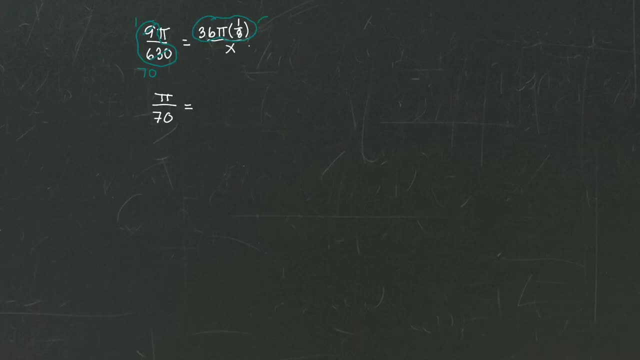 I'm going to take this little expression. I'm going to take this little expression here: 36 pi times one-eighth. So I have 36 times pi times one-eighth, but I'm going to write it with the eight in the denominator right. 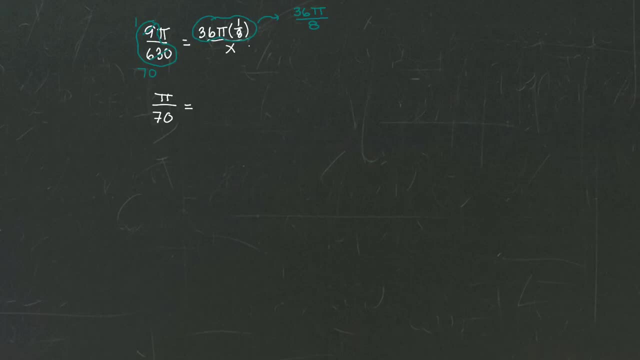 Because 36 pi times one-eighth is just 36 pi over eight, And again I'm going to cancel. I notice that four divides into 36 nine times and four divides into eight two times, So my numerator is actually just nine. 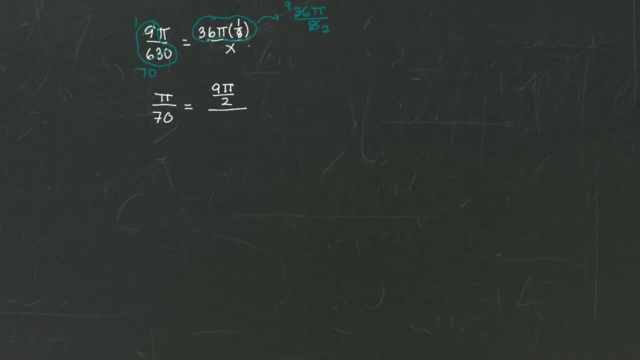 So I have 36 pi over two divided by X. Now I could go one more step and simplify this complex fraction, but I think I'm going to stop there To finish solving this proportion, what we need to do, or one method that students like. 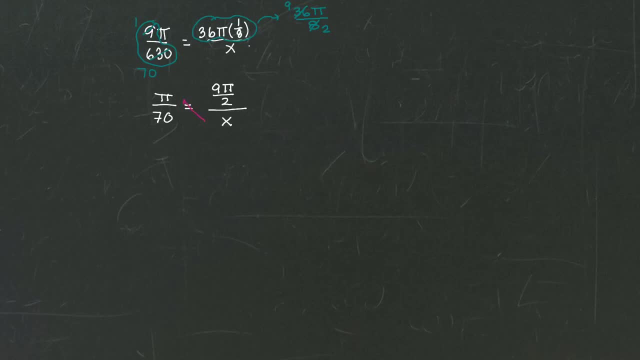 is the cross multiplication method, meaning we multiply across both ways, across the equals, and then we divide. So let's multiply across the equals, So we have three times three equals, which gives me pi times X equals, and then nine pi over two times 70.. 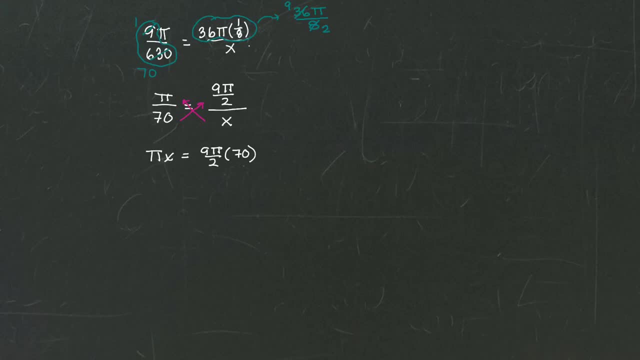 On the right side notice. I have one more cancellation. I can do Two divides into 70, 35 times, And so I have that pi times X is equal to nine times pi times 70.. So I have that pi times X is equal to nine times pi times 70. 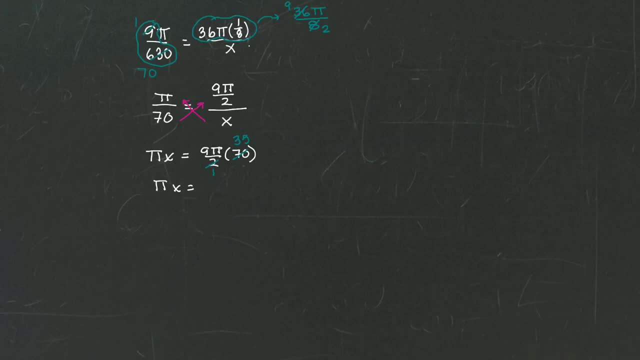 So I have that pi times X is equal to nine times pi times 70. So let's take out our calculator: nine times 35, and that gives me 315 pi. Now what is pi? Remember? pi is this irrational number. 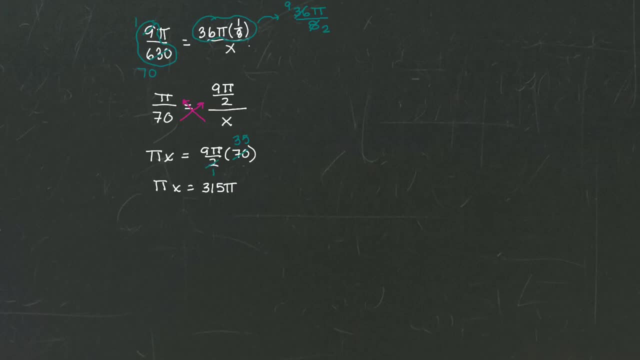 It's about 3.14, but it's not exact. Because it's not exact, I want to keep working with it till the very end and make my approximation at the end if pi still results. But if we notice, if we observe. 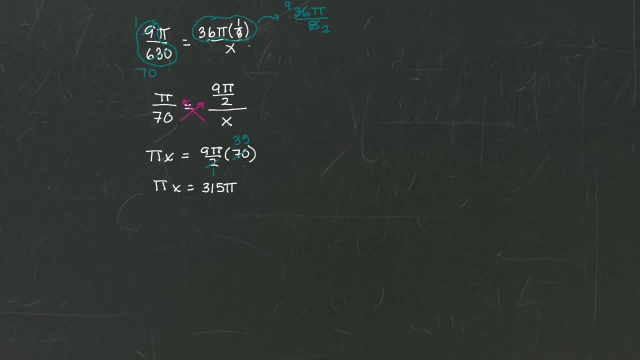 one last step to the right. one last step to solve for X is that we have to divide both sides of our equation by pi. Now, it's just a number, so we can do that. So we divide both sides by pi. But that makes it really nice because the pi disappears on both sides. 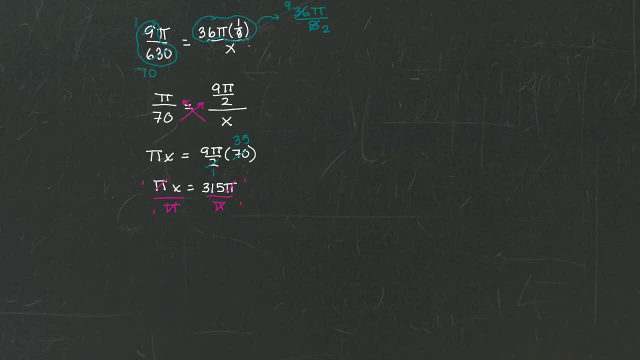 and we don't even have to worry about it. That tells me, then, that X is equal to simply the number 315.. X is just a number Plus 315.. Now how does that fit into our problem? What on earth were we trying to solve to begin with? 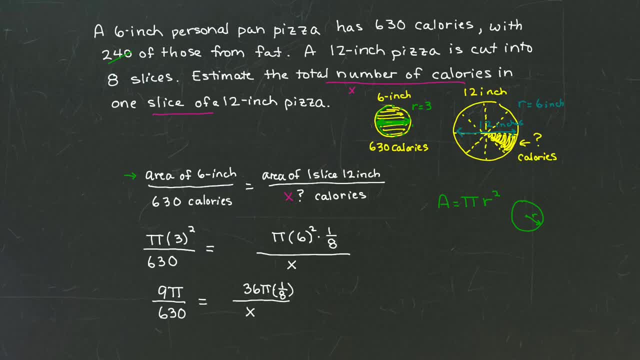 Well, let's go back. We found that this proportion solved down to give us that X equals 315.. And what was X representing? X was representing the number of calories that corresponds to one slice of 12.. That's the total number of calories in a 12-inch pizza.